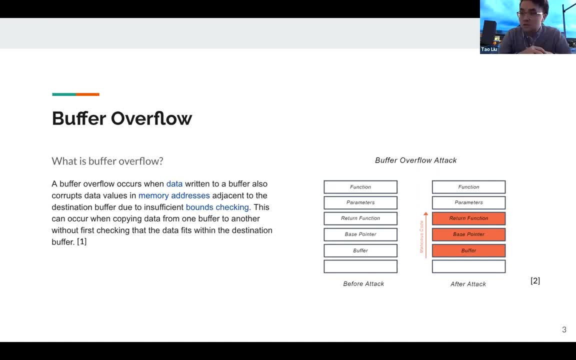 the attendees, So I will give a brief introduction. So yeah, I got the definition from the Wikipedia. So a buffer flow occurs when the data related to a buffer also crops data values in memory address that's adjacent to the destination buffer. due to insufficient bounce checking, This can occur. 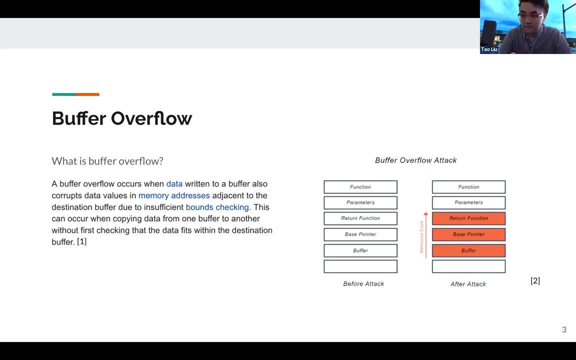 when copying data from one buffer to another buffer without first checking that the data fits within the destination buffer. So, as you can see from the figure, this is the buffer flow attack. So imagine, before the attack you have a buffer and after the attack you can see if you input something. 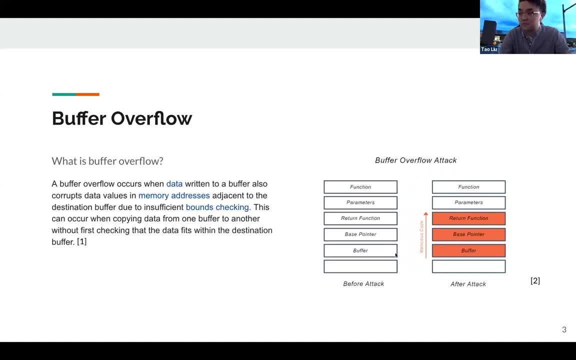 whose length is more than the boundary of the buffer, it will exceed the boundary and override the address space outside of the buffer. And this is how the problem happened. because you know in in the computer system the address. you cannot manipulate the address space randomly, because everything should follow its definition. 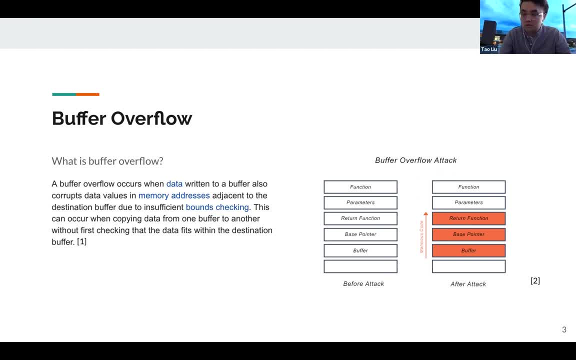 So if you cropped the address space outside of the buffer and then you run it the same way in the simulation program and you know policies. so if you randomly craft some memory in your computer, then usually a segmentation fault will happen and also the attacker can exploit such 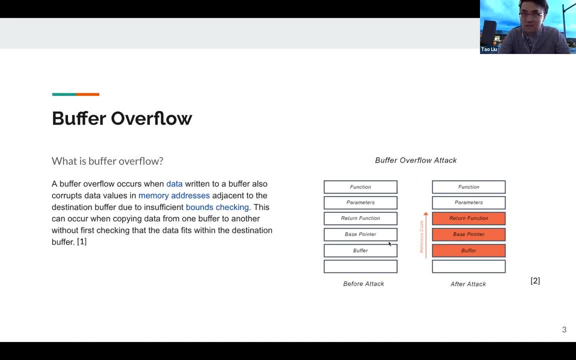 you know, opportunity to inject some malicious code to reinstall some worms. I believe 30 or 40 years, I think 40 years. So a lot of researchers investigate this issue and invent a lot of defense methods to protect the buffer, protect the stack and heap. 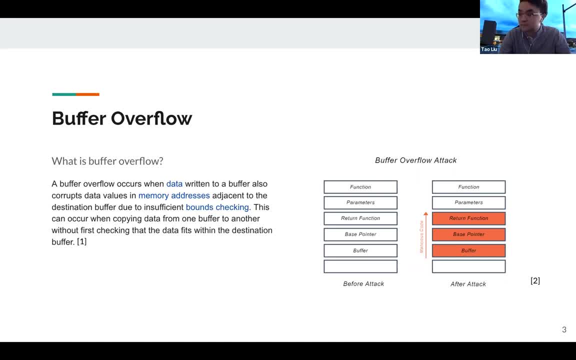 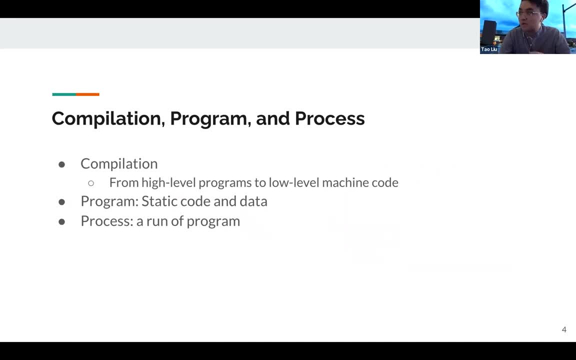 So yeah, basically this is a concept of buffer overflow And let's go here. So, by the way, if you have any question, I believe you can raise your hand. I think our coordinator can coordinate the questions and I can answer once I got a chance. 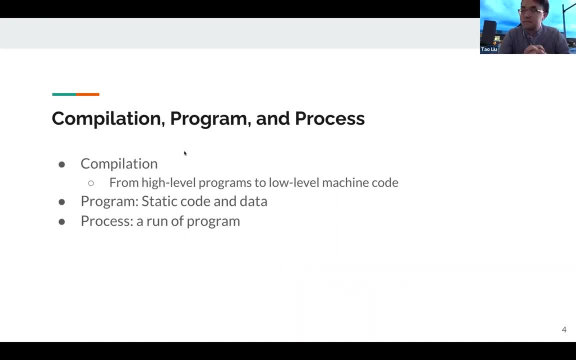 So firstly, we got to know some concepts about the program. So I suppose you have some experience with C programming. So we have the compilation. So the compilation will compile the high level program, like C, into low level machine code. Basically it's a binary code: zero one, zero one. 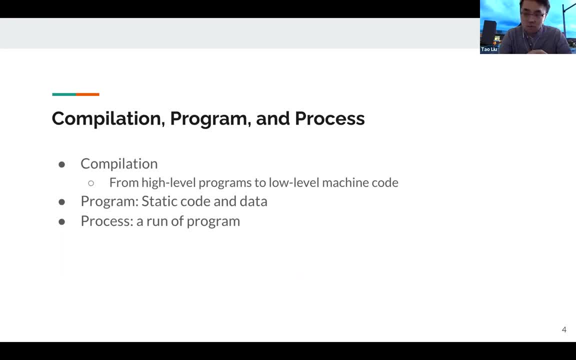 That is compilation. And what is a program? A program consists of static code and data. So the code basically is your program logic encoded in binary code, and the data: some constants, some global variables, local variables, So data. So this is a program. 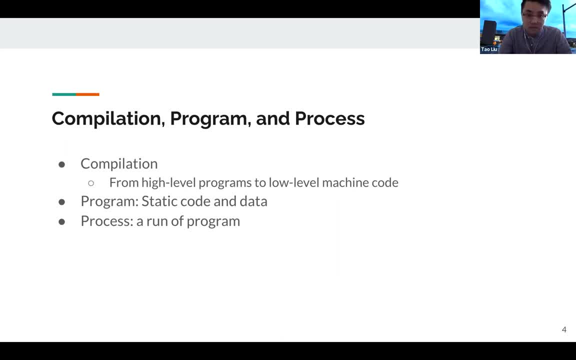 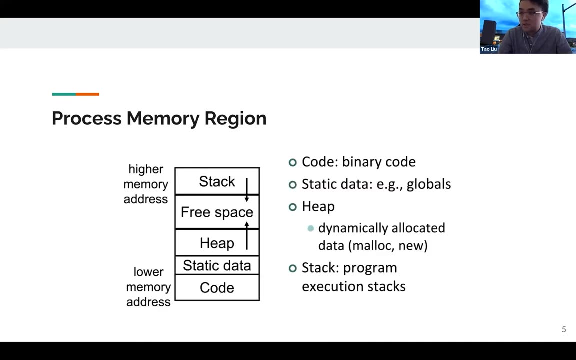 And the process is basically a run of program You want. after you compile the C code, you will get a binary file and then you want to execute the binary file. Basically, that is a process. So after we have these three concepts, we can go to the process. memory region. 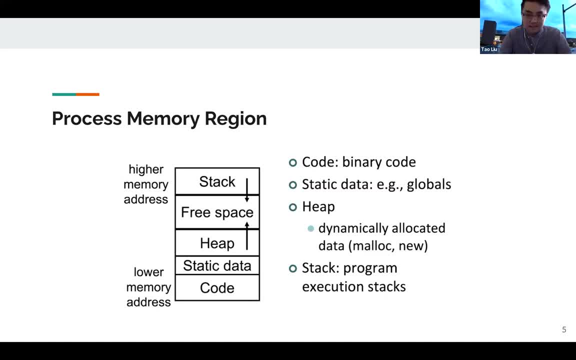 because, like I mentioned before, every process has its own memory region And the memory region should be protected very well. People can not randomly, you know, added or manipulate the address space. So basically, we have we- so this is a process- memory region. 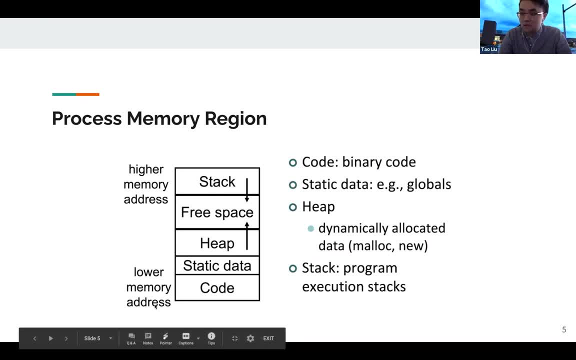 So here is the higher memory address and here we have the lower memory address And we have these components: the code, what I mentioned before, binary code And static data, for example the globals, And we have heap and the stack. 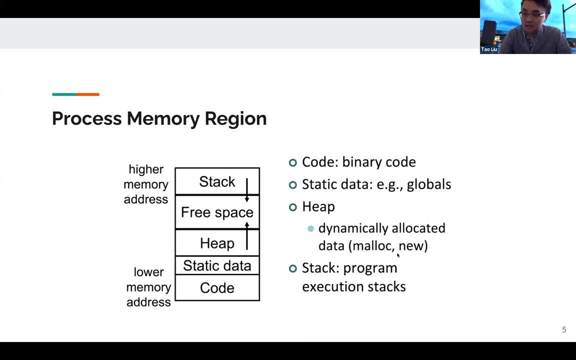 So the heap is the dynamically allocated data. So if you program with C you will mallocate or new some some memory space for your program And the stack is the program execution stacks. So this is the focus today. We are basically trying to know, you know. 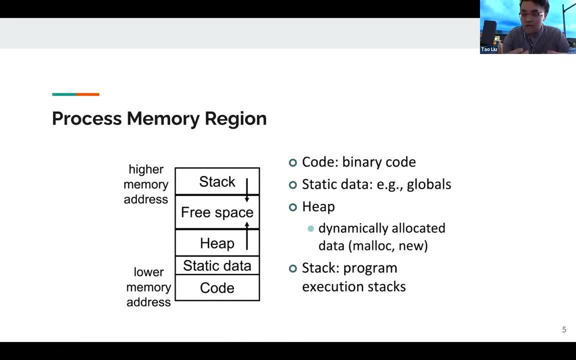 how to run the program, So how the buffer flow happens in within a stack. So this is a stack and this is the heap, And usually the static data and the code is in there at the end of the binary code And we have the heap and the stack. 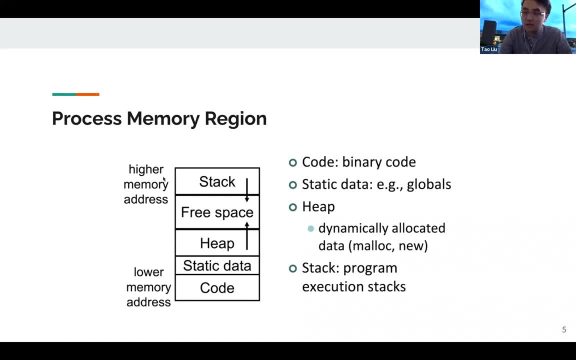 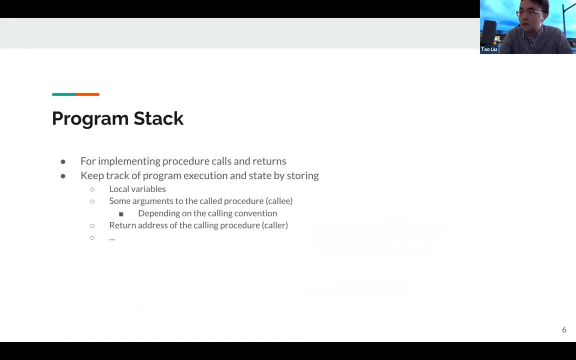 Basically, the stack will grows from the higher address to the lower address and heap will grow from the lower address to the higher stress And in the middle we have the free space for, you know, the memory usage. And then we are gonna see what is the program stack. 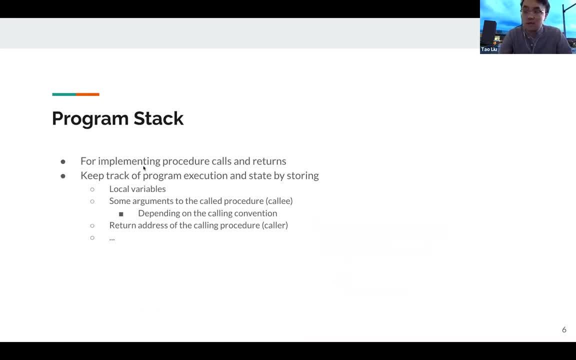 So basically the program stack is for implementing the procedure codes and returns. I have a figure later here, but first let's introduce the concept of stack. So the stack is used to keep track of program execution and the state. So the stack is used by storing the local variables. 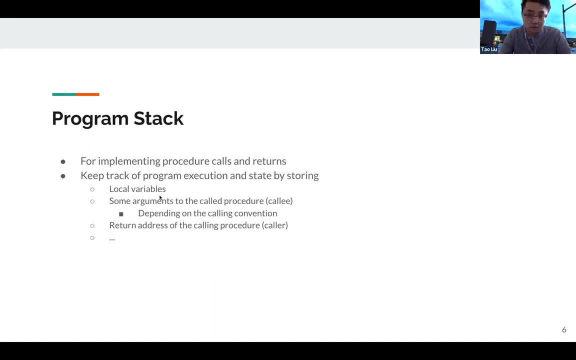 So you will define a lot of local variables in your C program And some arguments to the code procedure. So see, you have a main function and you have some functions to be code in the main function And the code procedure is the functions to be code. 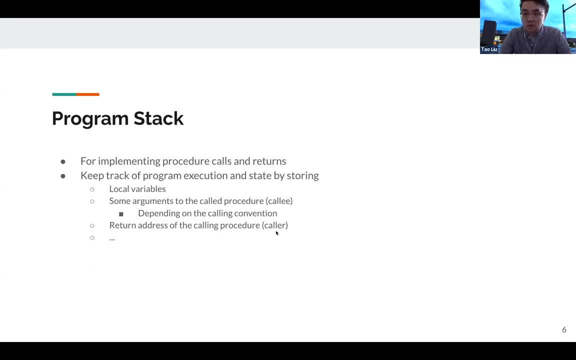 That's the callee And the main function will be the caller And also the return address of the caller will also be stored on the stack because after you finish executing the code function, you will need to return to your main function to execute its original execution order. 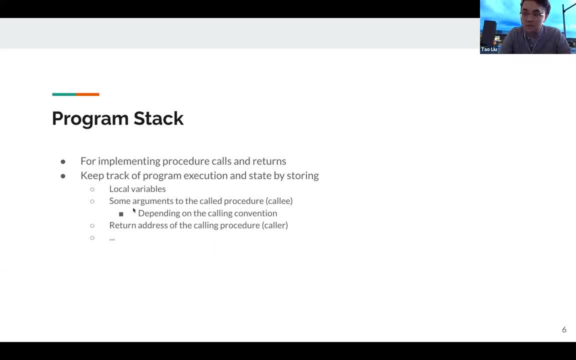 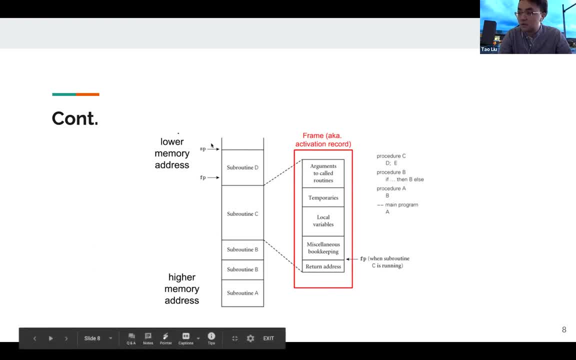 we have the main program A and it will create a stack for this whole program And, for example, the main program, code A and the procedure A, code B. So the B will be the callee and the A will be the caller, And if we continue this procedure, 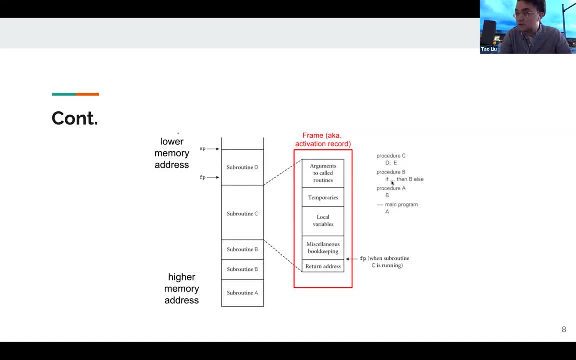 we continue B, for example B, and then B will be the caller, And if a conditional statement, then B, and, or else I think here should be a C, So else C. So if we execute the C, it will be the subroutine C. 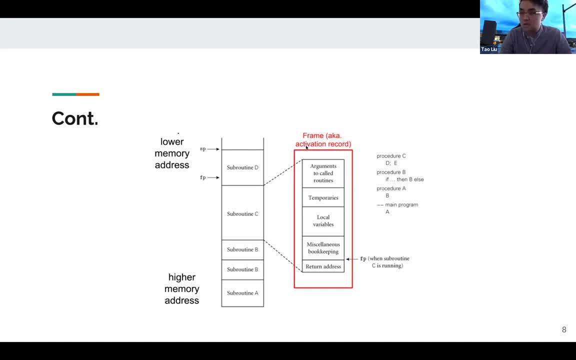 And then we will go into this stack frame, which is also acknowledged as the activation record. Actually, this is the currently live stack frame. This is what you are currently executing. This is what you are currently executing. This is what you are currently executing. 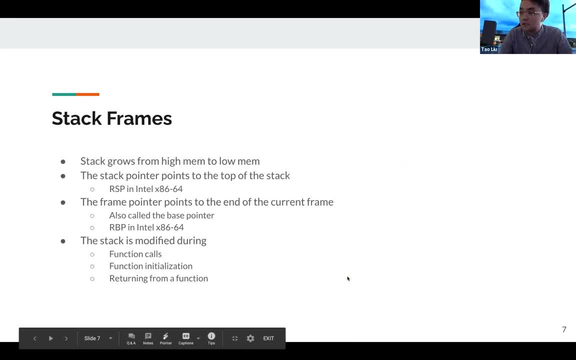 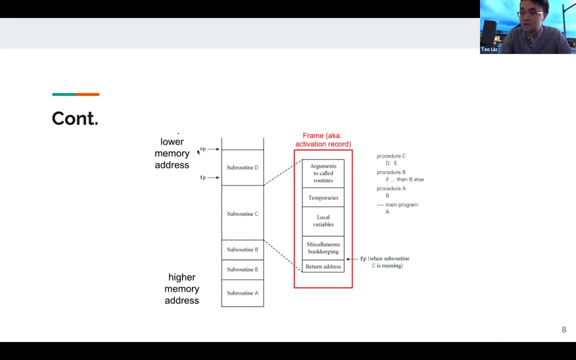 So this is the stack frame And let's see the stack grows from the higher address to lower address And we have the stack pointer. The stack pointer will point to the top of the stack. So here, as you can see, we have the stack pointer. 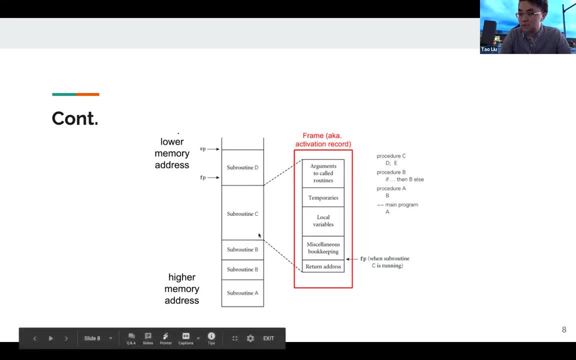 So the stack will grow from the A, B, C and the until D And the stack will point it to the top of the stack. And the stack will point it to the top of the stack. It's the subroutine D, And then we have the frame pointer. 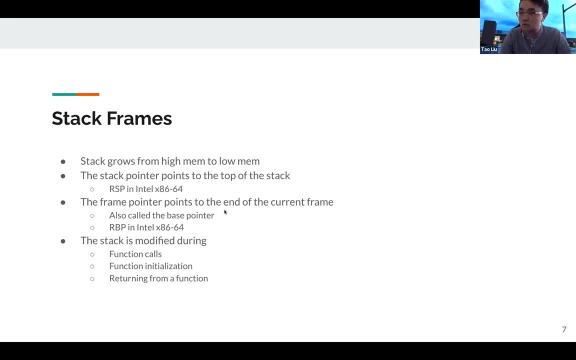 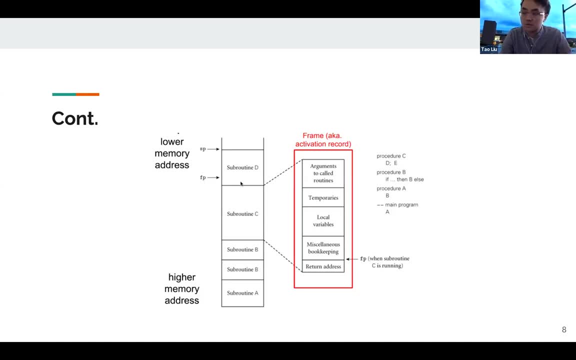 points to the end of the current frame. So you can see in this figure this is a frame pointer. It will point to the end of the current frame. Actually, this is just an example figure to show the activation record If the frame pointer points to here. 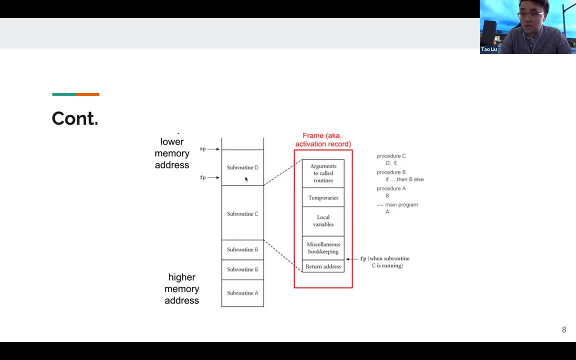 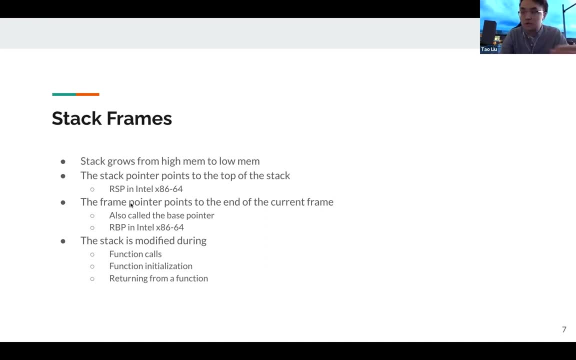 then this one should be the current activation record. So yeah, this is a frame pointer. So we have a stack pointer to point to the top of stack And we have a frame pointer point to the end of the current frame, And then the stack is modified during some procedures. 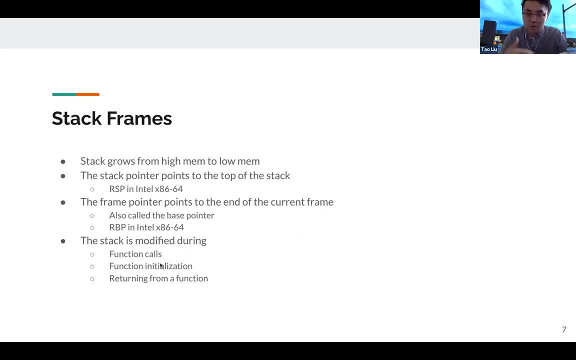 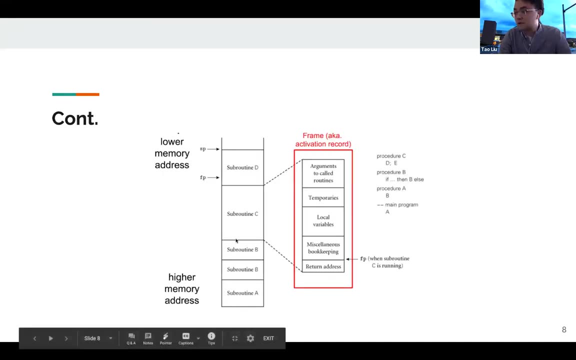 One of that is the function call. We will try to call some functions, But there is a function initialization and also returning from a function, So I will illustrate them one by one later. So yeah, this is the. so now you have a big picture of what the stack is. 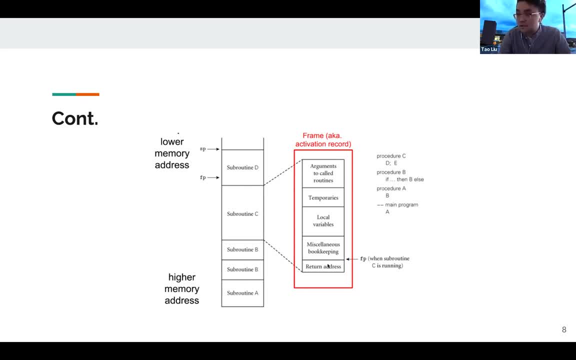 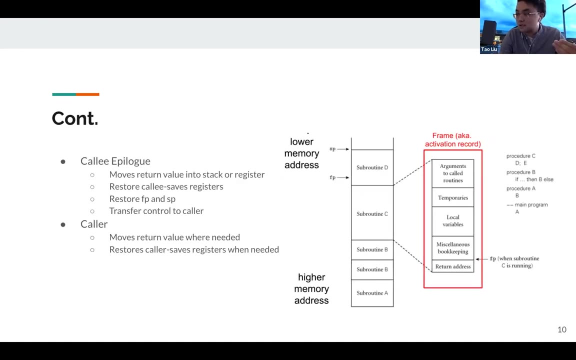 and what a stack frame is. And, as you can see, in the stack frame we have some components, We have the arguments to code routine. I think this is many. this is more conceptual. Let's see in the code here. So we have the main function. 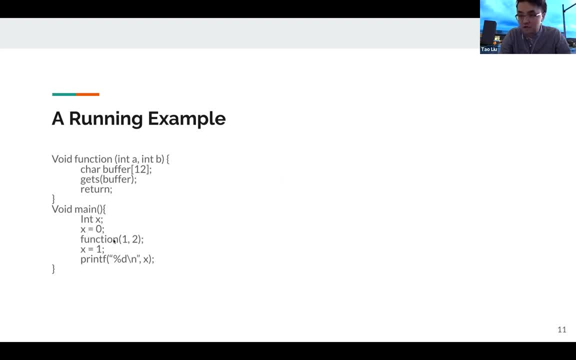 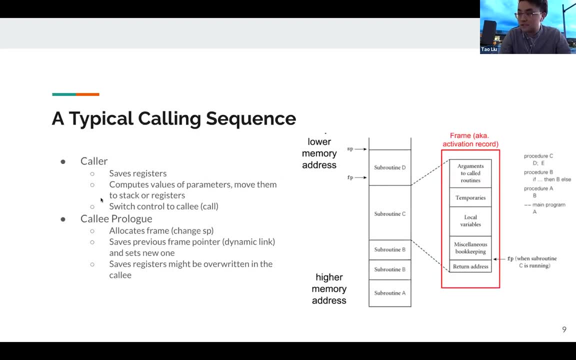 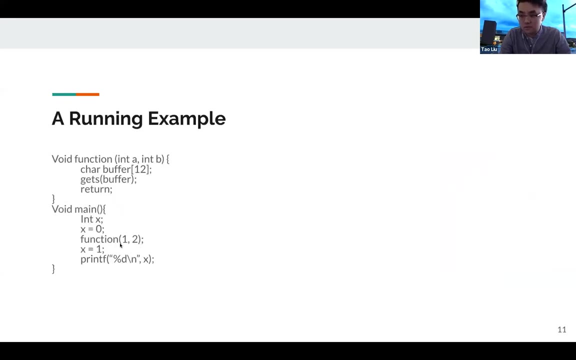 and in the function, we will call this function. Name the function: We will call this one. And, for example, based on this figure, arguments to code routine, which will be these two: These two are the arguments to be passed to the function. 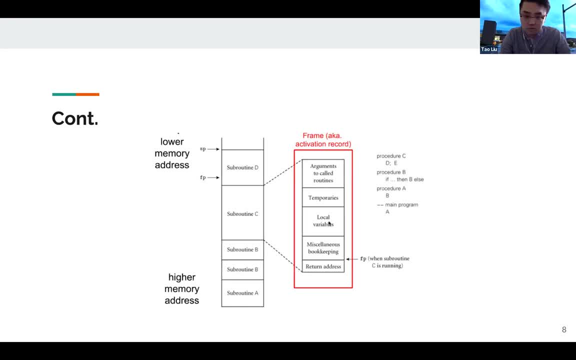 And then we have the local variables which you define in your functions, And also we have the return address. The return address. so still remember I said, after you execute this function C, you will come back to B, right, So you execute this one. 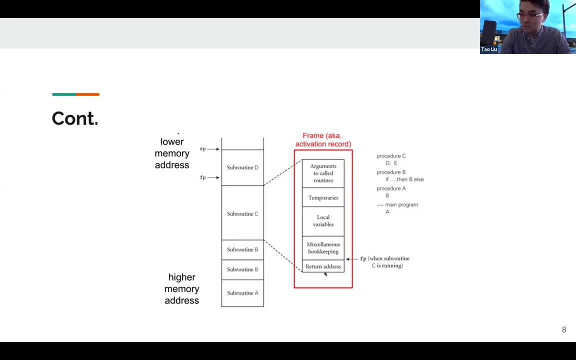 this one will be killed and it will return to B, So basically the return address will store the address of next instruction to be executed. So this is how. this is what the return address is, And basically the buffer overflow vulnerability will be exploited by manipulating the contents. 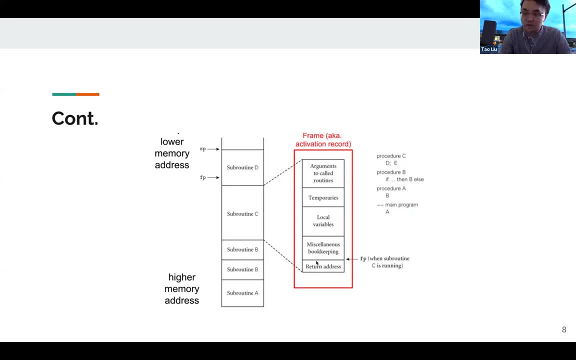 of the return address, Because basically you can. if you can manipulate the contents of this address space, then you can control what the next instruction to be executed is, And then you can control the program. So this is the concept: how the buffer overflow vulnerability can be exploited. 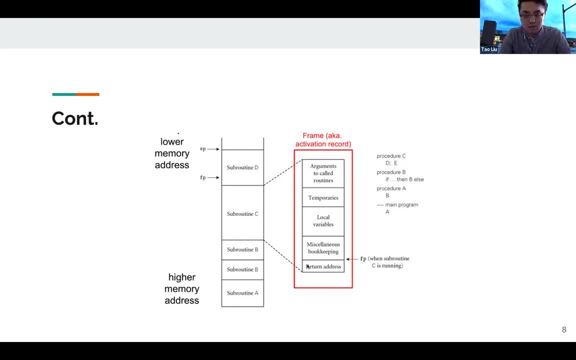 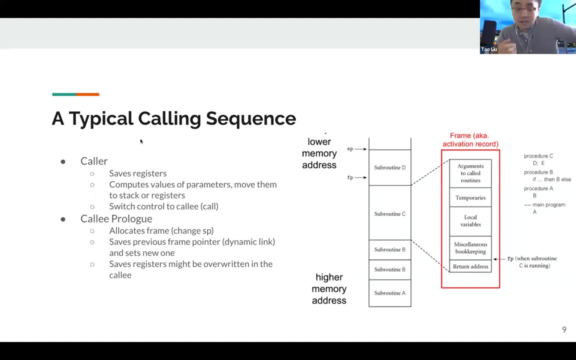 So this is the key, And then later on we will see how this one can be manipulated or overwritten by the buffer overflow vulnerability. So we need to, before we, before we, can understand how the buffer overflow vulnerability can be exploited, we need to know what a typical calling sequence is. 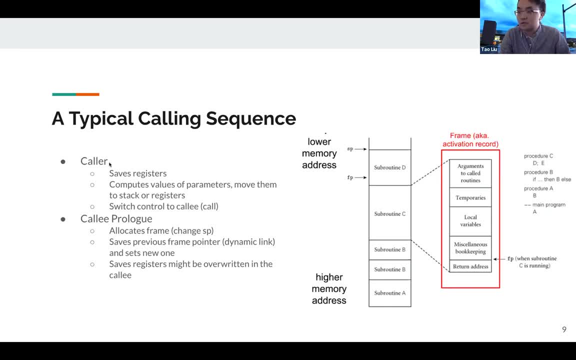 So still the same figure. we have the caller. So let's focus on one example. So we have the caller, caller B, the subroutine B. So we have a caller B and the callee should be the subroutine C. So the caller will say: 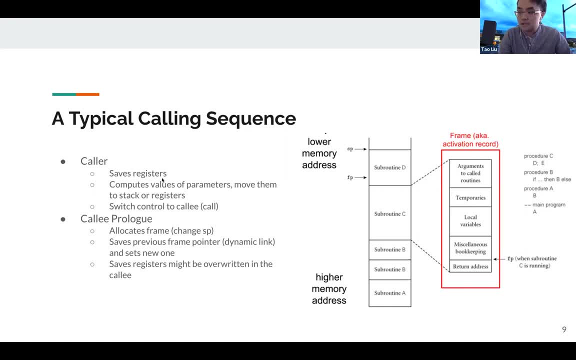 Hello B, So I can use the той uma code, The graphical name C in the, to say hey, could you please run talk? It's my question. can you please run the talk? the contents of the register can be erased or can be used for the new function. 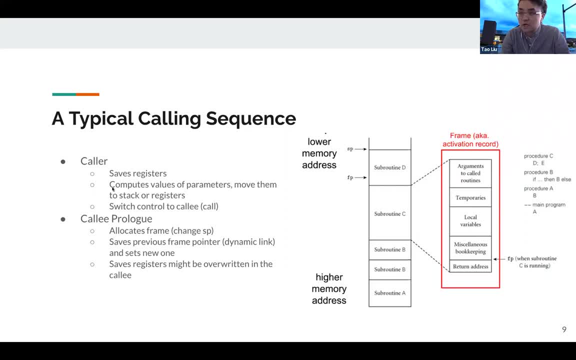 So the caller need to save registers and also compute the values of parameters, move them to stack or registers for the use of callee, And then you need to switch the control to callee because you will need to execute the callee function And during every function call. 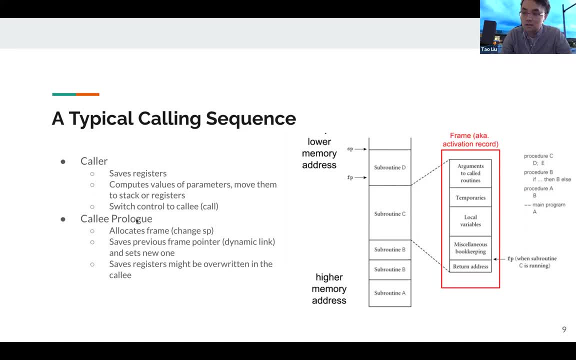 there will be a callee prologue. So this is also a classical definition in the computer science textbook. So the callee prologue. okay, Yeah, the callee prologue will basically allocate the frame. So you need to allocate the frame for the callee C. 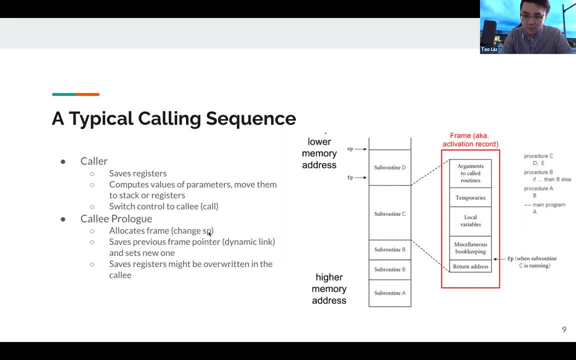 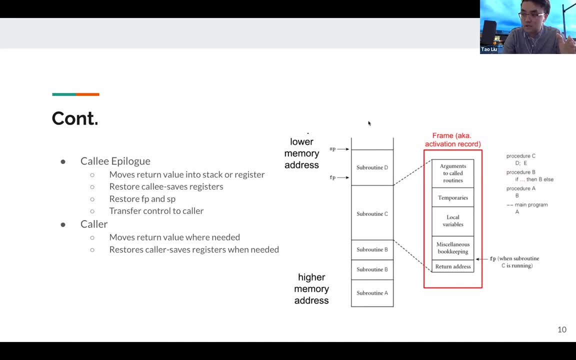 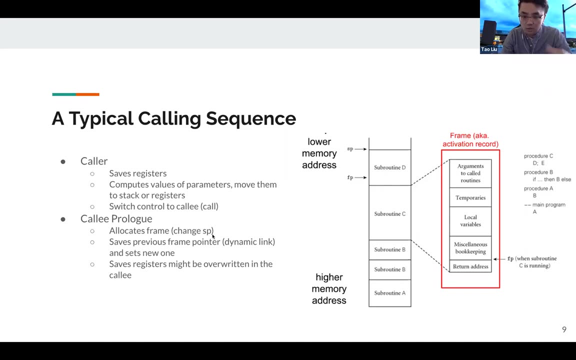 and then you need to change the stack pointer, because you create a stack pointer and then you need to add a new frame. So the address space has been increased, has been increased to the lower memory address, So the stack pointer will point it to the top of the stack. 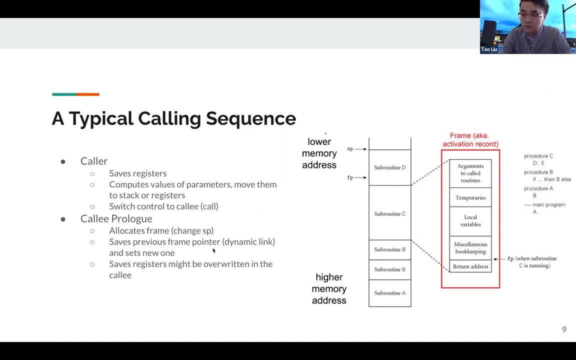 And then it will save the previous frame pointer and assess new one, because previous you are. previously you are executing the subroutine B, So the FP, the frame pointer, basically will point it, basically will point it to the subroutine B, So the FP, the frame pointer, basically will point it. 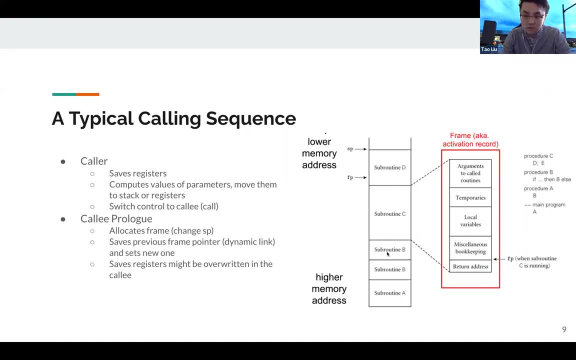 to the end of subroutine B. However, now you are trying to execute the subroutine C, So the frame pointer will point it to the end of the frame of subroutine C And also, in the meantime, the old frame pointer will be stored, as you can see. 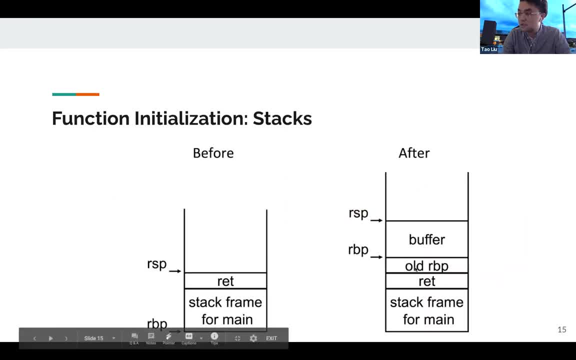 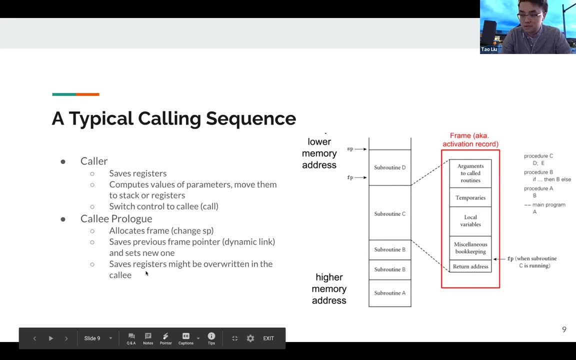 in later. yeah, the older frame pointer will be stored so that later on you can restore the. restore the previous function And then let's see, Yeah, it will. it again will save some registers. might be overwritten in the coli, So it will save the registers. 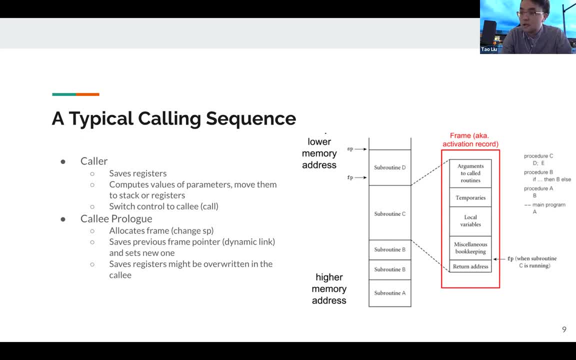 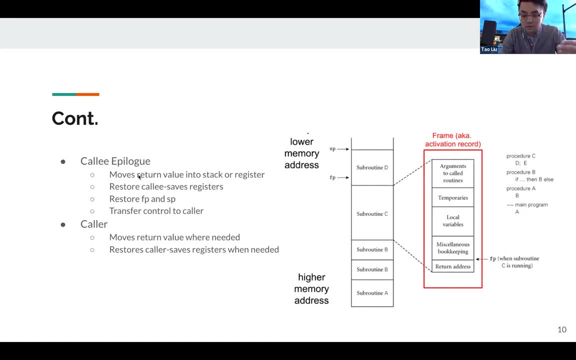 for the sake of the caller function. And then we have coli app log. This is what happens when you have already executed the function C, You want to return B. return to function B. So in this app log it will move the return value into stack or register. 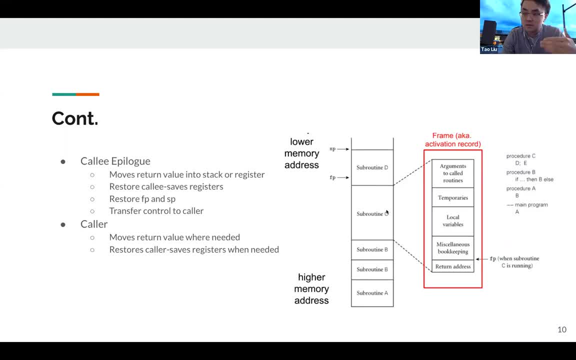 So you execute the C and then you have something to return to the subroutine B. So you will move the return value into stack or register for the subroutine B's usage And then you will restore. the coli saves registers, So you remember the coli. 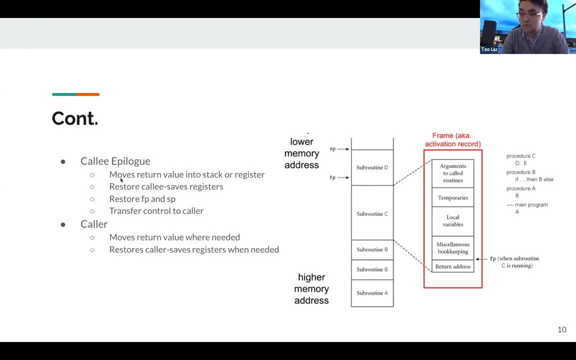 Save some registers. So it will, it will restore them And also it will restore the frame pointer and the stack pointer, because now you have finished the execution of subroutine C, So you will destructor or queue the stack frame And then you will need to change the frame pointer. 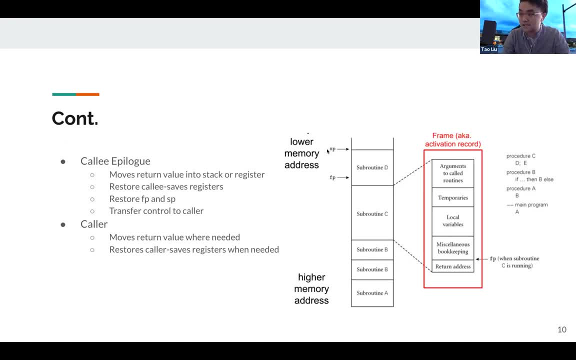 to point to the subroutine B and also the stack pointer. Basically it will move from the top of here To the top of subroutine B, So it will restore the frame pointer and the stack pointer And then it will transfer the control to the color. 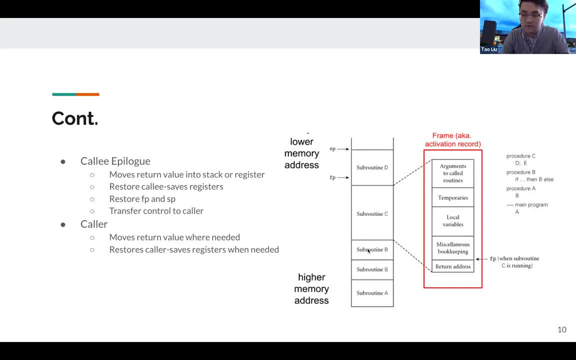 to the color B And you know everything will start from the B again, And so the color will move the return value where needed and restore the color saves registers when needed. So this is a very high level when needed. So basically it will follow the program execution logic. 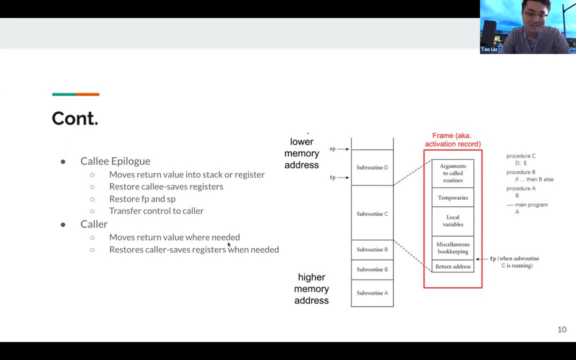 So I can only use the when needed to, you know, to show the high level concept. So yeah, let's see. Is there any question here? Okay, You've seen memory over Or other data structures, Oh, okay, So you can. 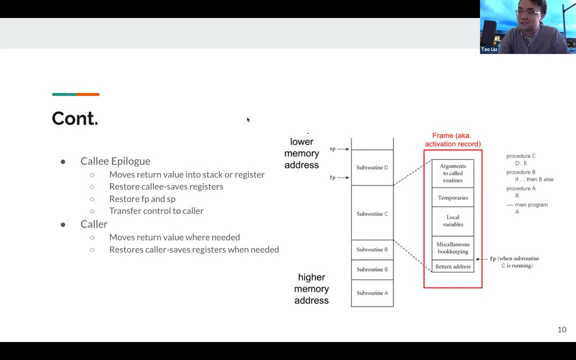 you cannot just think this is a how to say, Yeah, this is an interesting question. I actually currently I do not have a clear answer for that, But as you can see, the stack is. I think this is. give me a minute. 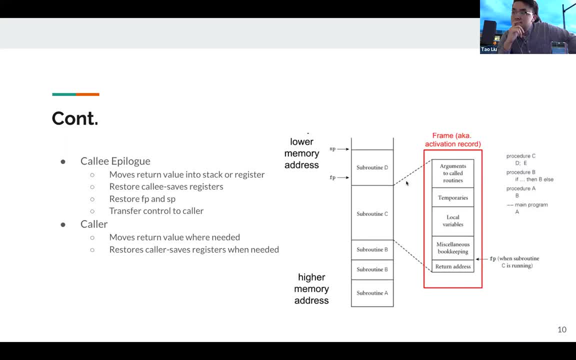 Actually, I think this is not the stack We are usually actually. this is not the stack. Maybe I took, maybe it is, Maybe I took it really using in our programming. So this stack is basically more related to the system design. 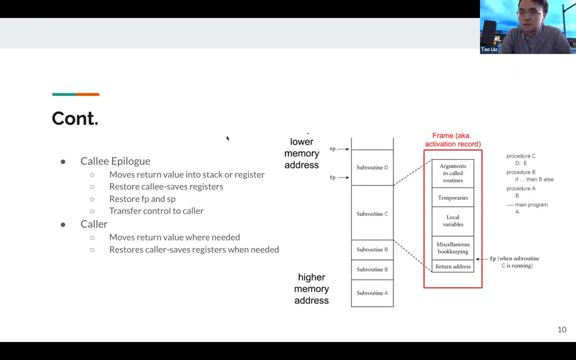 And actually I cannot give you a clear answer for now, but I'm sure you can search it and see whether you can get any helpful answer online. Yeah, but I think this is a classical design of the system. There must be a lot of investigation and research on this. 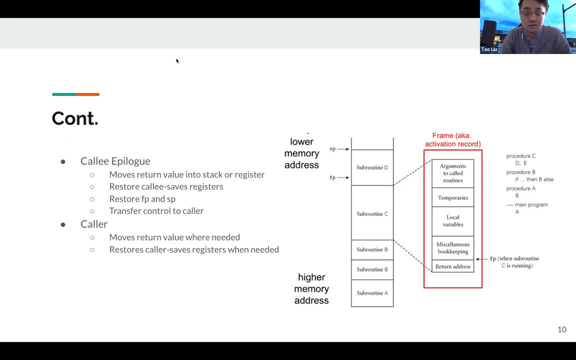 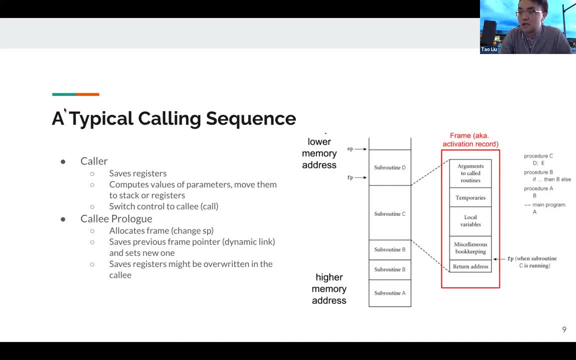 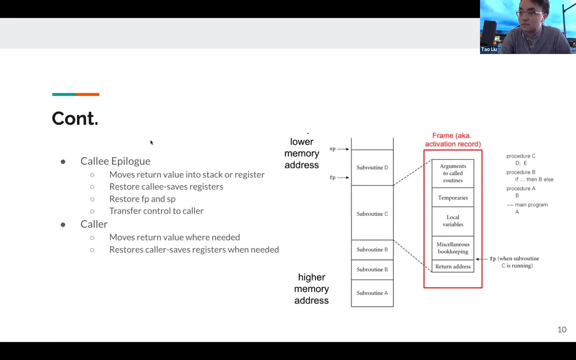 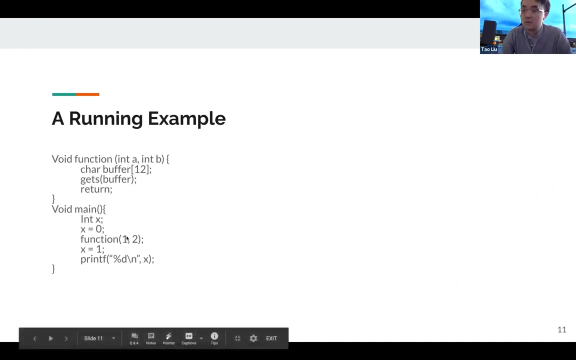 Yeah, sorry for that, But it's still a good question. And then, so now we have the, we have, you know, we have our understanding of the typical calling sequence And now we can move on to a running example. So this program is very simple. 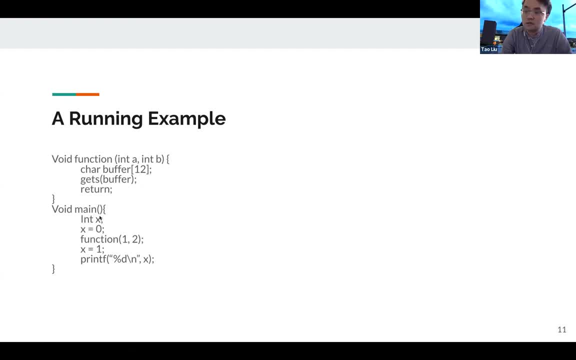 We have the main function and the way. we have a integer X and we gave it zero and a way call function And we give the parameter one and a two and the program will go into the function. And I see we have a buffer here. 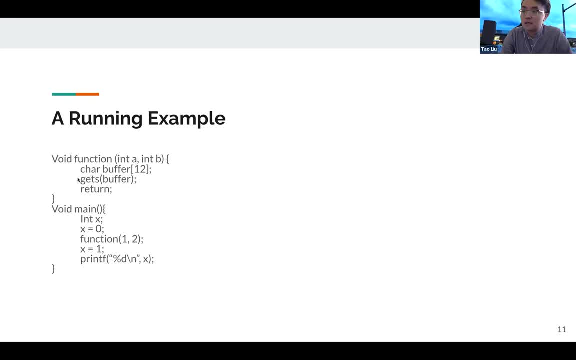 and it has the lungs of 12 bytes And the program use the gas function actually, which is a very dangerous question. dangerous function because it does not check the the boundary of the buffer. So if you, for example, if you input like 20 bytes to it, 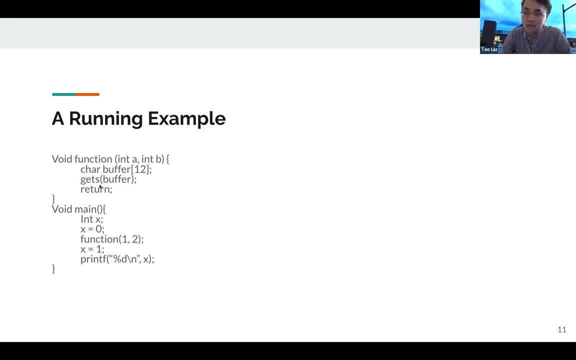 it basically will accept all the 12 bytes, And that is the problem. So the 12 bytes will override the memory space. I will show you a small demo later to show how it works in detail And then it will return. So it will return and execute. 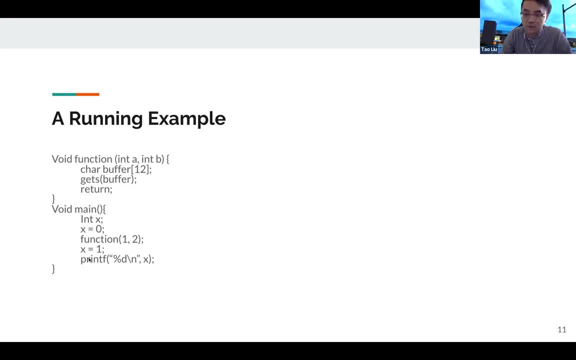 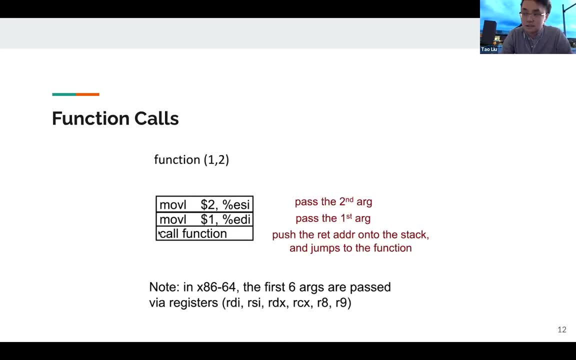 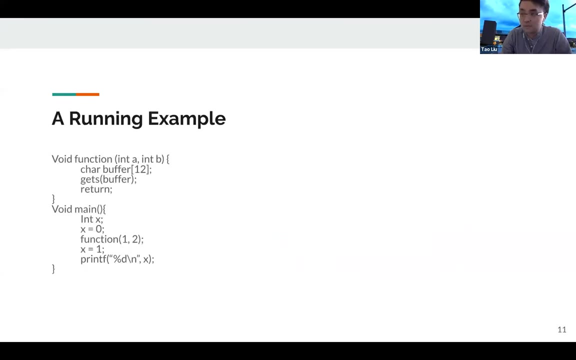 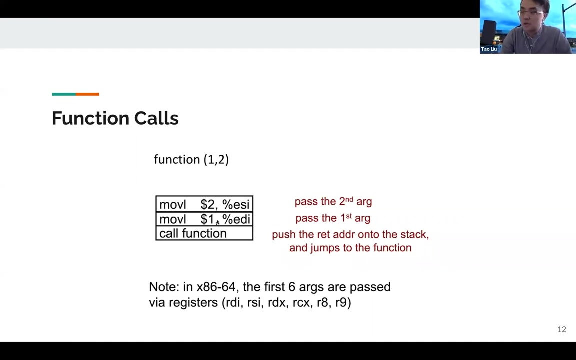 Execute, the X is equal to one and you want to print out the X. So this is a very simple example And let's see how we can apply the former definitions into this simple example. So we have function call, It calls the function and it has a parameter one and a two. 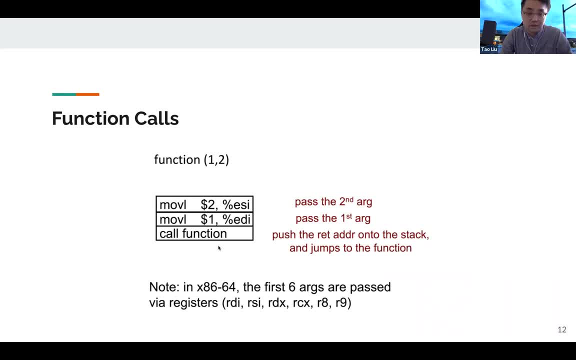 And in the assembly code. I believe you, if you have some experience, when we use the GCC to compile the code, we can get the assembly code before we compile it into the machine code. So this is the assembly language assembly code. 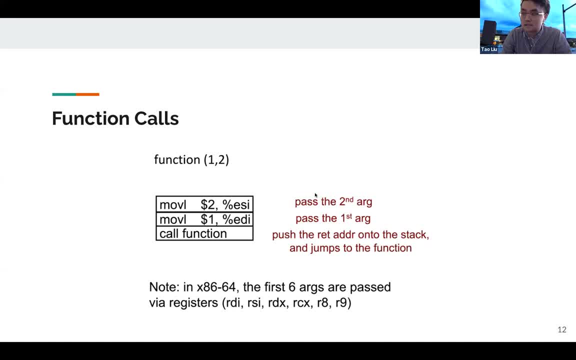 So basically these two instructions to pass the two arguments into the registers and use them in the call function, And then it will call the function to really execute the function. so in the same time it will push the return address onto the stack and it jumps to the function. 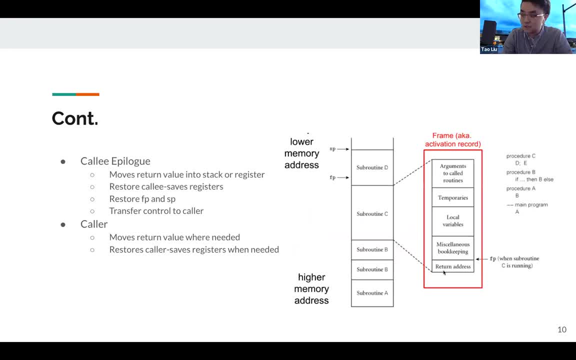 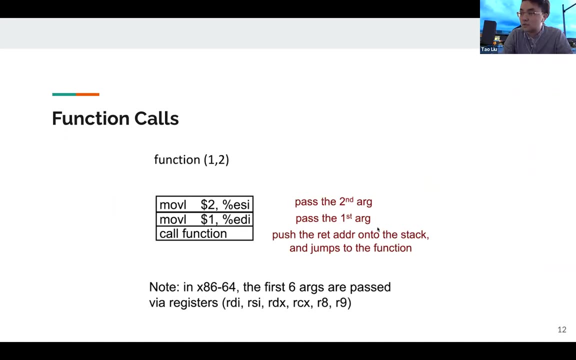 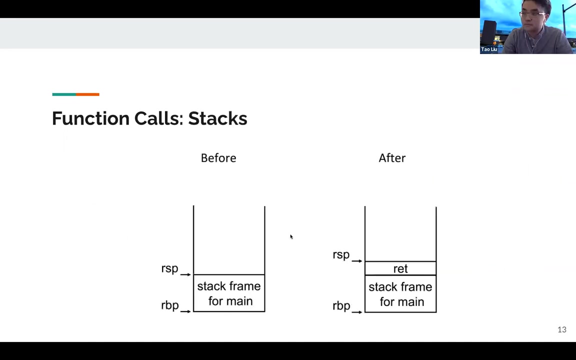 So still remember the return address, right? So it will put the return address into the stack. The return address is the next instruction you will execute after finishing executing the function C. So it basically will push the return address onto the stack And this is the function call. 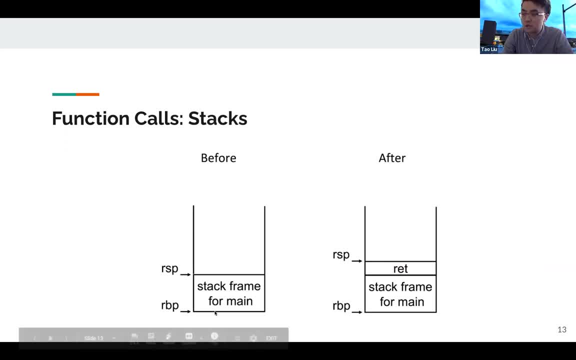 And this is how the stack will change during a function call. So this is the frame pointer points to the stack frame for main. And this is the stack pointer points to the top of the stack. And then, after you execute the function call: 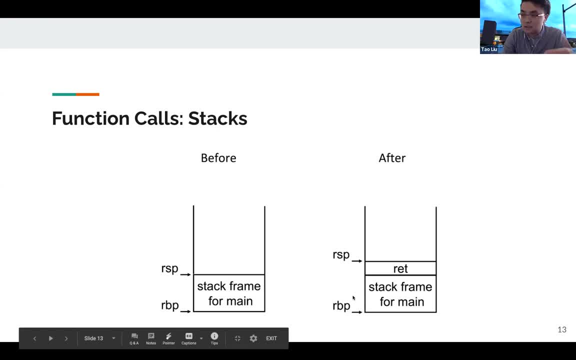 the stack frame currently because it does not execute the call function yet, so it will still point to the, the stack frame for main. And the stack pointer has been increased to the to a higher address because you have already created the return address to store. 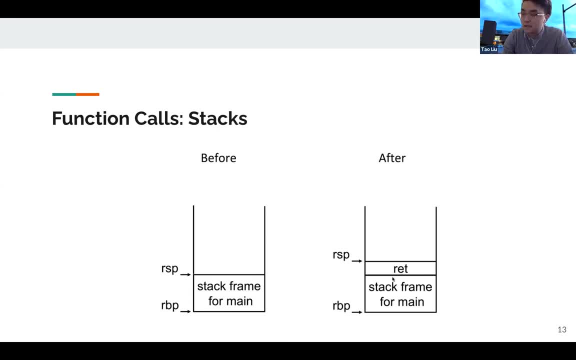 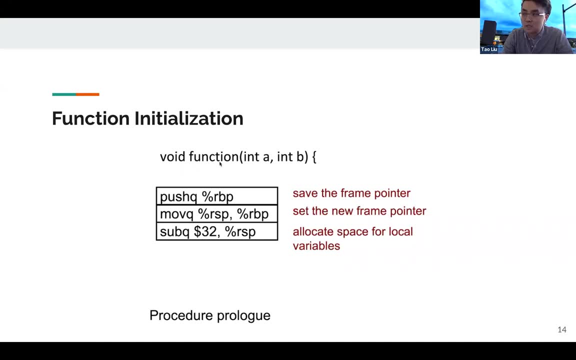 the next instruction you want to execute And this is the function call, And afterwards the call function will do the initialization. So in this procedure it will save the old frame pointer And also it will set the new frame pointer and it will allocate space. 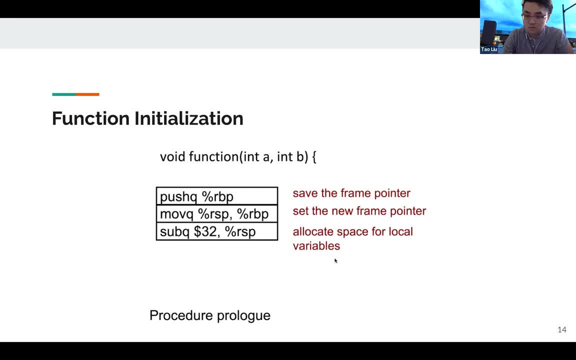 for local variables, because we, when you create a new stack frame, you'll need to allocate space for the memory usage. So it will allocate the space for the local variables. Yeah, this is a function initialization and let's see how the stack change during this procedure. 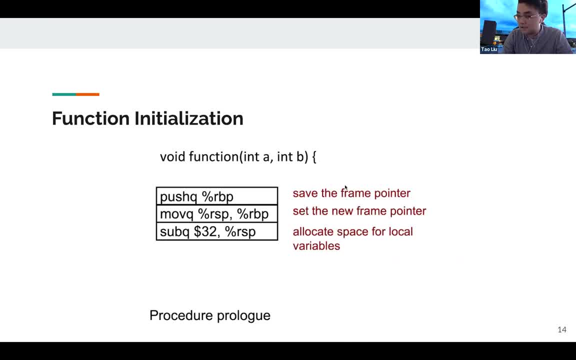 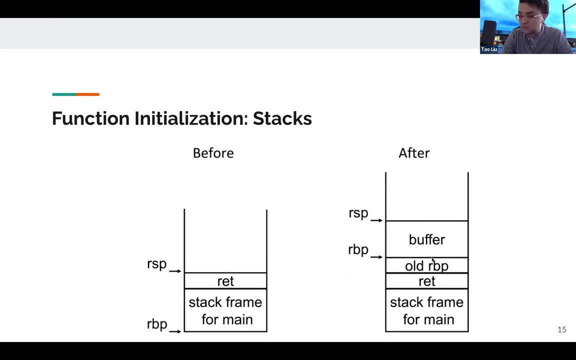 So, as we can see it, saved the old frame pointer, set the new frame pointer. So we can see it, saved the old frame pointer and set the new frame pointer to the end of the current active stack frame And the stack pointer will point to the top of the stack. 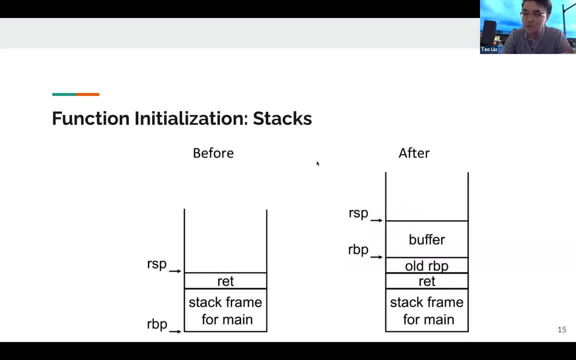 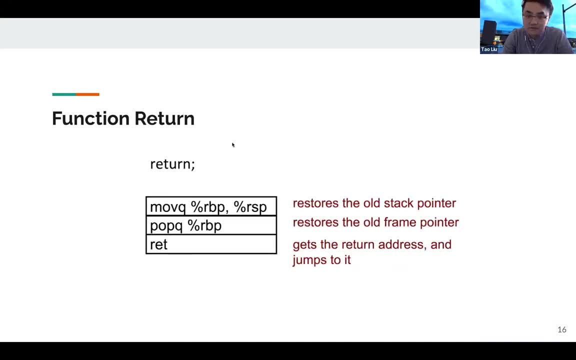 So yeah, this is how the stack changes during the function initialization, And then next is the function return. So after you execute the function, it will return. So it will restore the old stack pointer, because you are killing the current stack frame. 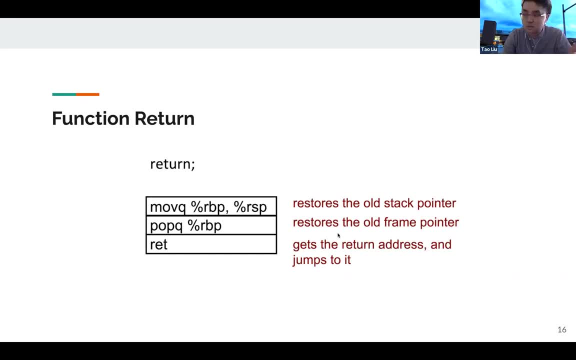 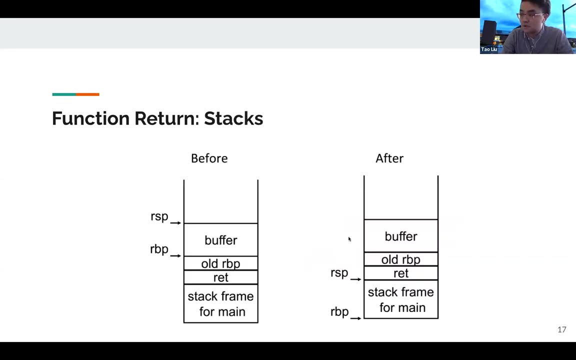 So it will restore the old stack pointer and also restore the old frame pointer and you get the return address and it jumps to it because that's the next instruction you want to execute. So let's see how the stack changes. So, as we can see, 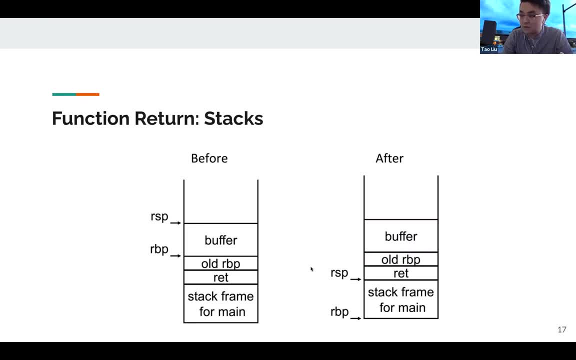 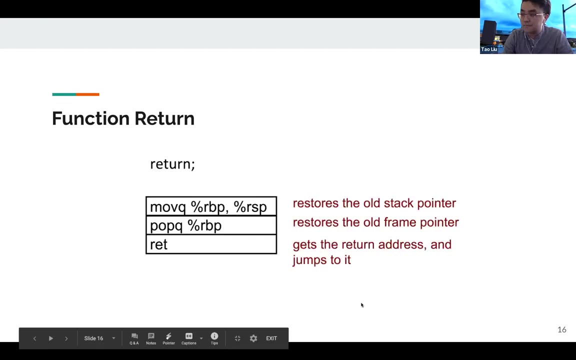 the stack pointer will change from the top of the buffer to the top of the stack frame for main And the frame pointer will change it to the location to point to the stack frame for main. So this is how the return works during. this is how the stack changes during our function return. 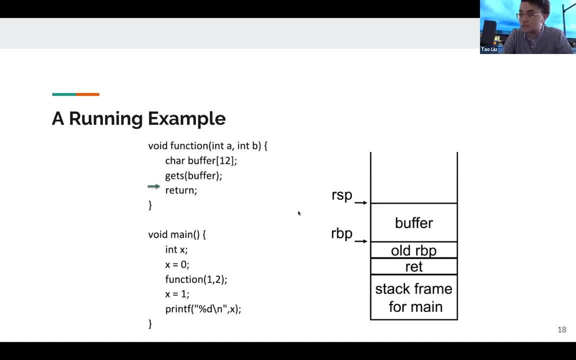 And then let's see. Okay, I think this is a time that, because now we have all the background knowledge about you know process, memory, region and how the function code works and what the coding sequence is. So I guess now we are ready to know. 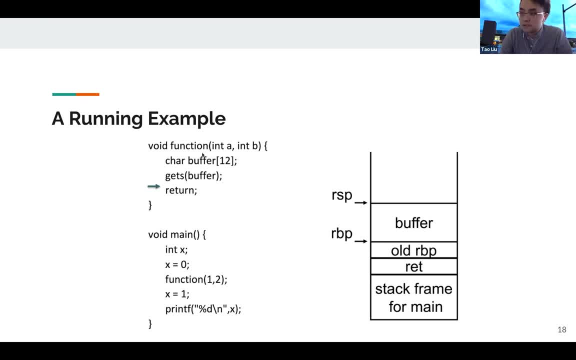 what exactly is buffer overflow? So, as you can see in this running example, as I point out here, when the program receive the input from the user, the user can give the input of any loss. However, you only have a 12 bytes of buffer. 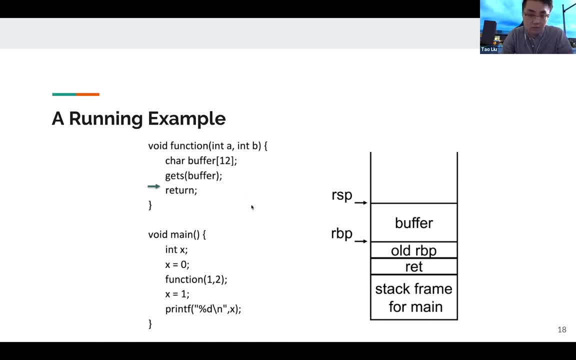 which means it will exceed the boundary of the buffer. And you can see the buffer is only 12 bytes but actually you can input like 20 bytes. So the stack will not increase to the lower address, So it will only the. 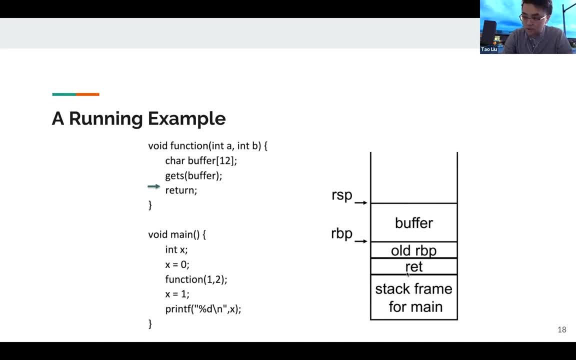 the input of contents will be only stored from the top to the end, which means you will override the return address. Of course it depends on the offset between the stack pointer to the return address, the location of the return address. So that is the tricky part. 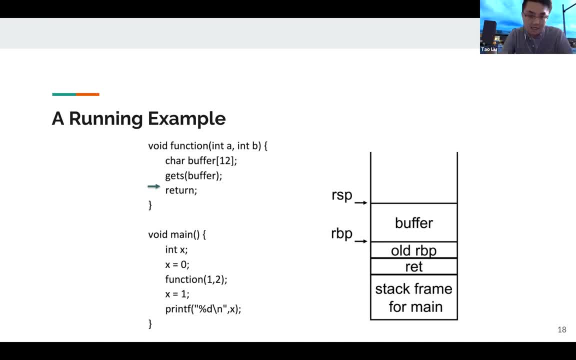 That is how the attacker need to calculate. They need to use some method to calculate the offset So that they can precisely know the location of the return address, and then they can precisely manipulate the return address to point it to where they want to execute. 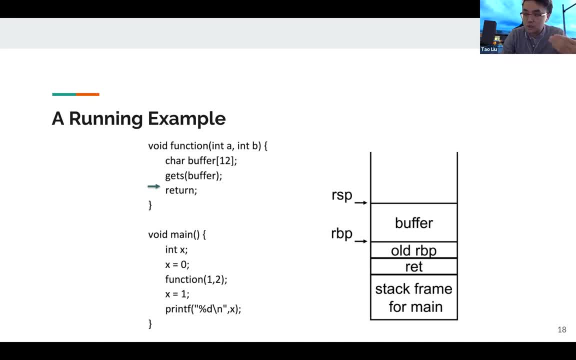 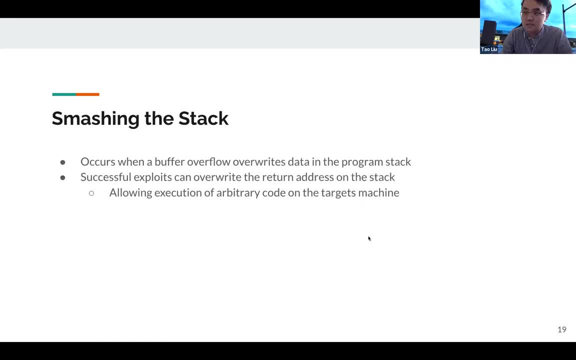 So before we move on to that part, to how to manipulate the return address, let's foresee what is: smashing the stack. So the smashing the stack is okay when the buffer of flow overrides they the data in the program stack. 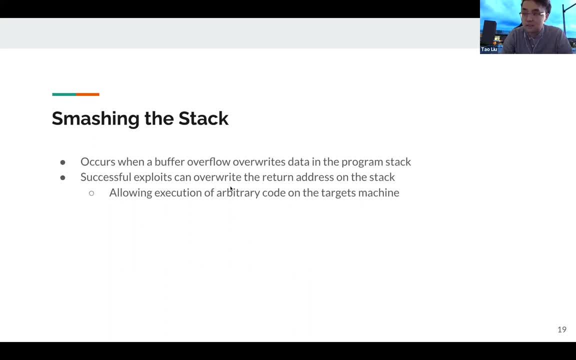 and the successful exploits can override the return address on the stack, Like I mentioned before, and it will allow the execution of arbitrary code on the target's machine. So this kind of arbitrary code execution is the most severe vulnerability in the, you know, CVE database of United States. 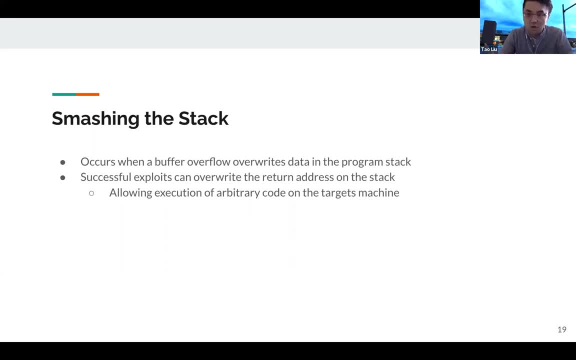 They all have a CVE database which stores all the vulnerability CVE IDs and the vulnerability type and the vulnerability details. So this is the most severe one in the database, because if your program can allow the execution of arbitrary code in the most dangerous scenario, 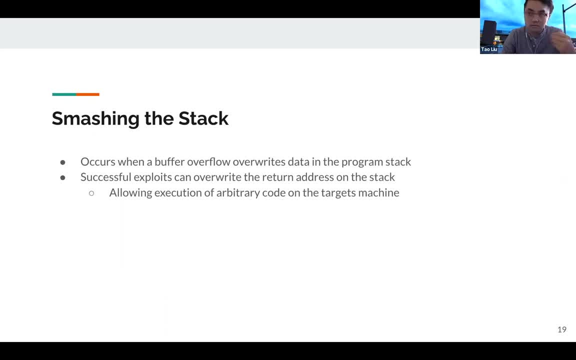 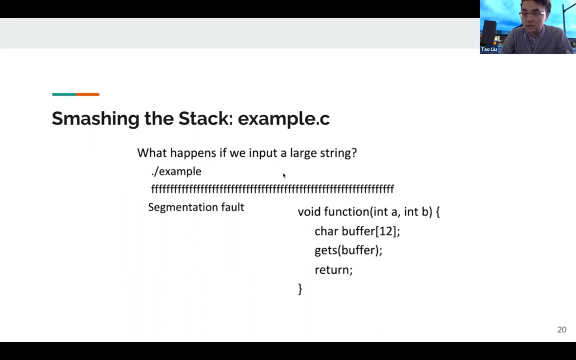 the attacker can obtain your root privilege village, which means they can execute any code, they can install the worm, they can take control of your computer, they can store your information. so this is the most dangerous one. and in the, in our example program, it's a very simple one and the logic is very simple. so what? 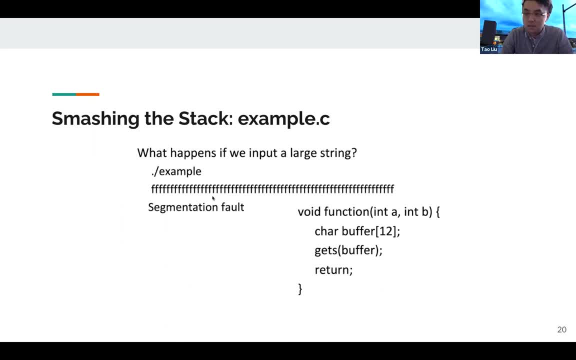 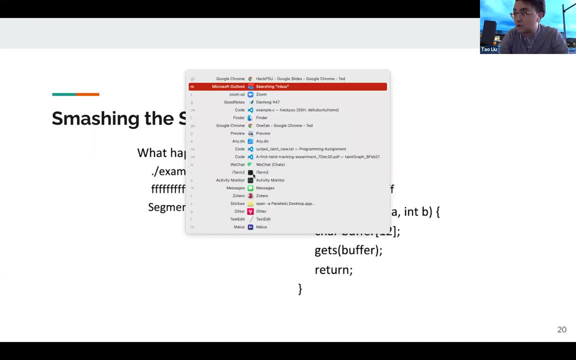 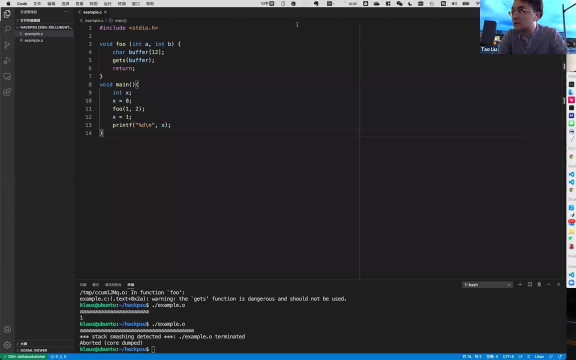 happens if we input a large screen, so it will cause a segmentation fault. uh, so i can show you a quick demo here. let's see. okay, so this is the, this is the program, uh, and then, uh, this is uh, the name is example c, and let's let's first uh, uh, let's first uh see. 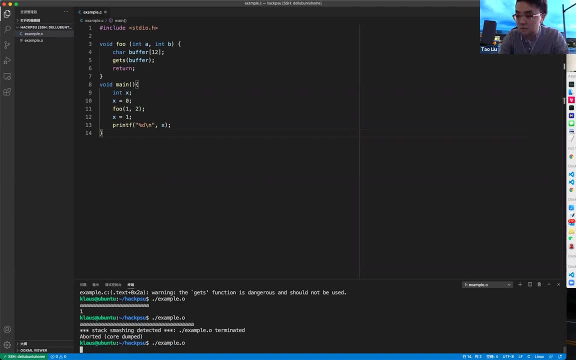 we want to execute this program and now it's waiting uh input. so let's give it uh, one character. yeah, so it successfully. you can see here, it successfully output one which is the right output, because, following the logic, the right output should be one: the value of x. however, if we execute it again and let's see we give it a 20 a. 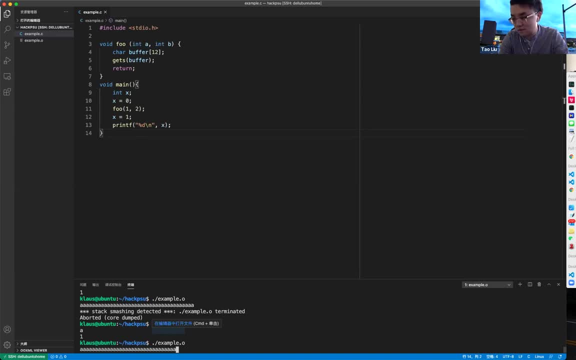 we give, we give it a you know much longer one, and then oops it, uh, stacks smashing detected. so basically, in the program in the current uh uh computer, it has the stack protection, uh, so basically it detects such stack smashing. so it will terminate the program. and if you use this, 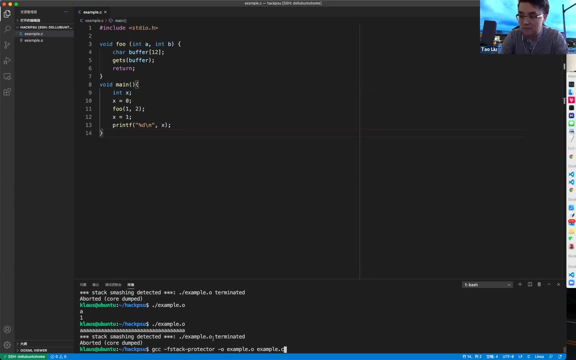 command to: you know, compile the code. let's see what happened. basically, this means you okay, wait a minute, so it should be this one, yeah, this one, the no stack protector, which means you do not, you disable the stack protection, and then you compile it and you execute it, and then you give it the you know dangerous input. 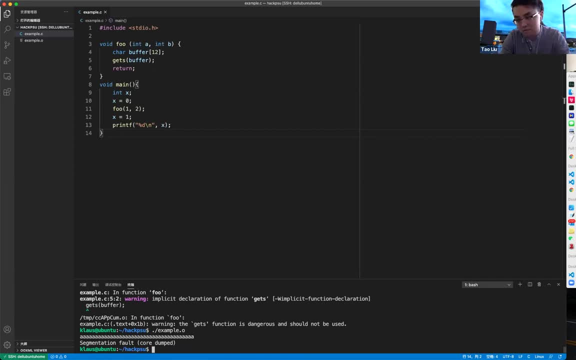 and uh, okay, this is another segment, okay, but uh, yeah, just uh, uh, let's ignore this part. but uh, if we, if we execute the code like before, and then we can see there's a stack smash here, stack smashing detected, so this is the uh, this is the uh, the part of the buffer overflow and what? this is what happened. the. 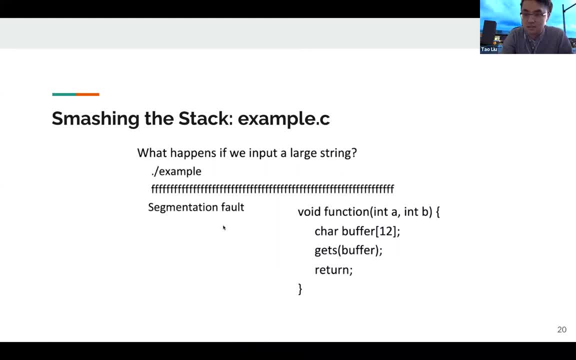 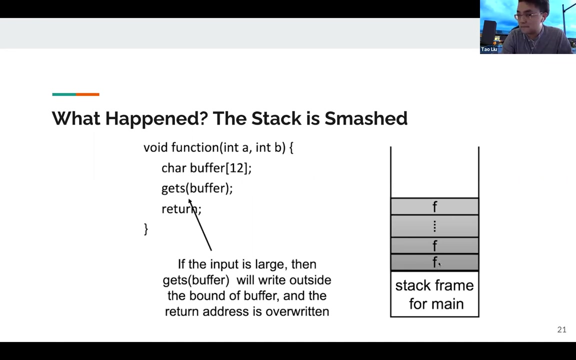 smashing the stack, but basically this is not very dangerous because the program will terminate itself, because counter computer system has already has the stack of protection and it will prevent such such smashing, however. so this is, this is the how the stack is smashed. so you can see. this is your input. 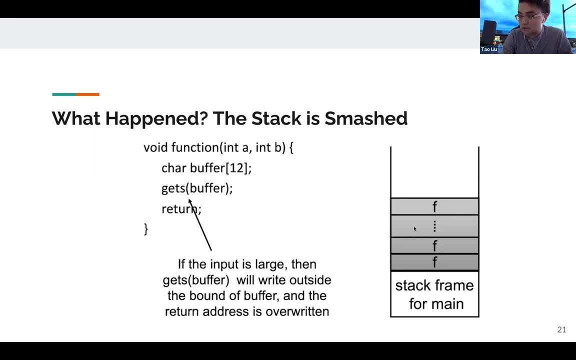 basically it will override all the contents and then so the input is large and then the buffer will write: outside of the bound of buffer and the return address is overwritten. so because your, your return address is already overwritten with some characters, so when you try to execute the 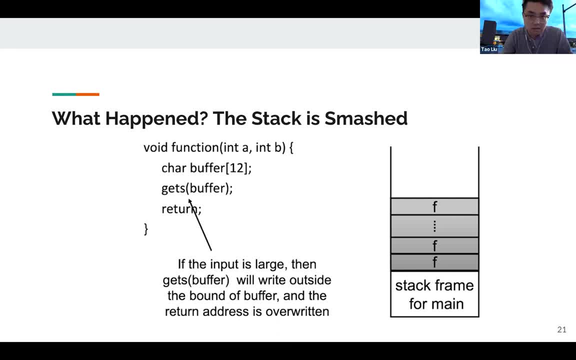 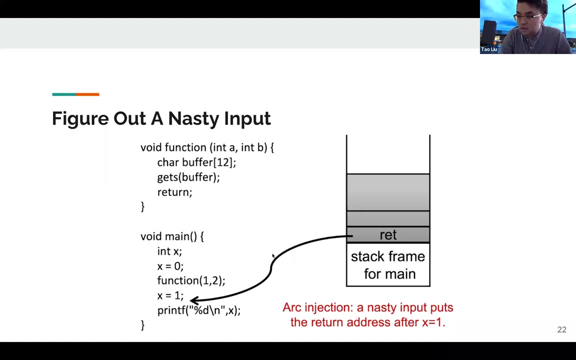 next instruction. it cannot be executed. so that's why the program will terminate, because the instruction is invalid, so your program cannot work well and basically this is the program crash. and let's see if we can figure out a nasty input. so, for example, we do not want to execute the x is. 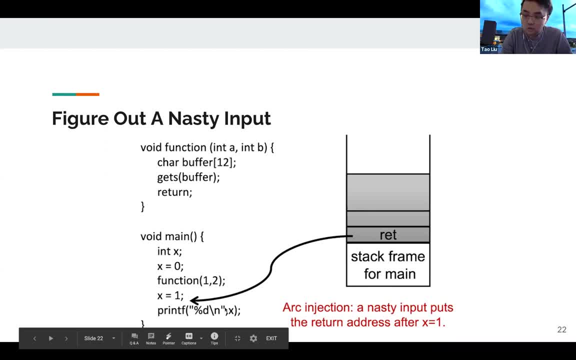 equal to one we want. the program can just print out: the x is equal to zero. how we can do that? so this is an nasty input and actually this is. yeah, this is something that i i plan to show, but you know, due to the time constraint, that i do not prepare that demo. basically, that demo will be. 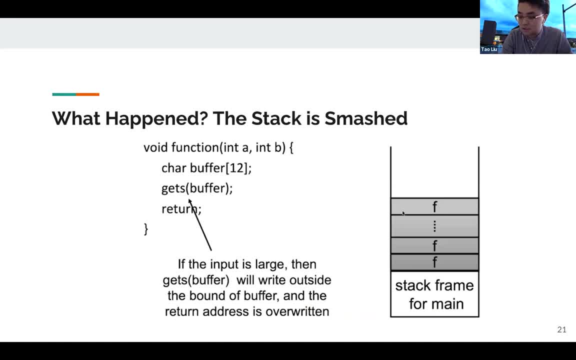 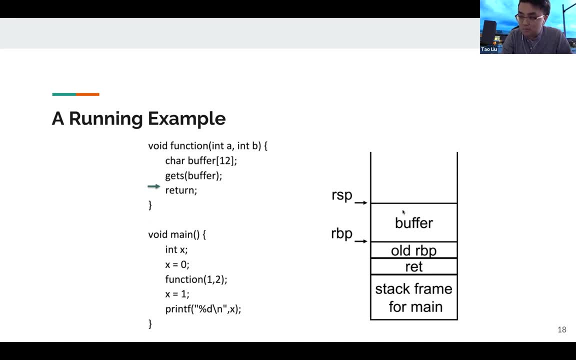 you calculate. you calculate the- i think this figure is better- you calculate the, the offset between the top qualities for the buffer and the top of the return address, And then you will change the contents of the return address and you want to manipulate that address space to something you want to execute. 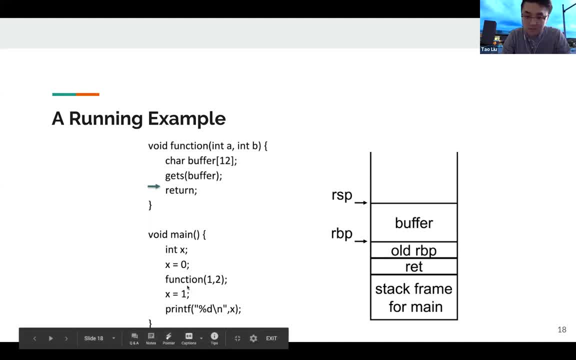 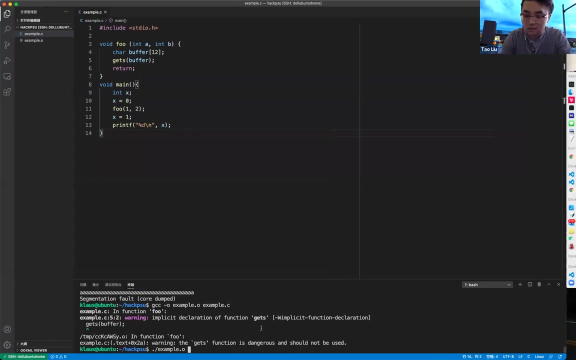 For example, we want to skip this assignment, So we will know the address of this assignment, and then we want to skip that part, skip that address. And this is more advanced materials. but I can show you the concept one. Let's see here. 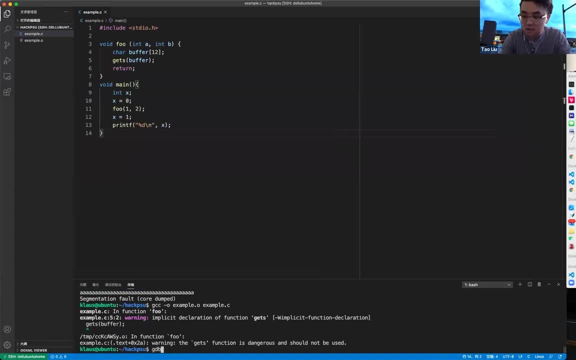 So we can use the gdb. gdb and basically the gdb is a tool to monitor your program execution. You can print out the stack contents and you can print out the register information. So let's run here. And there is a comment which is the example. 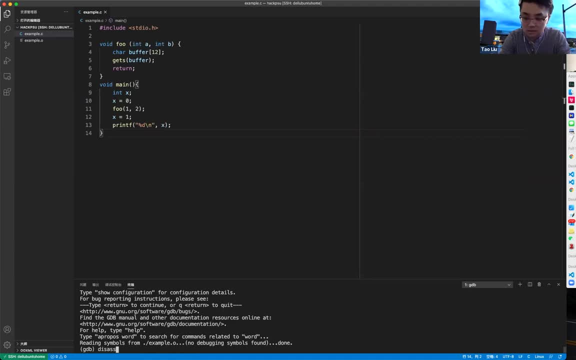 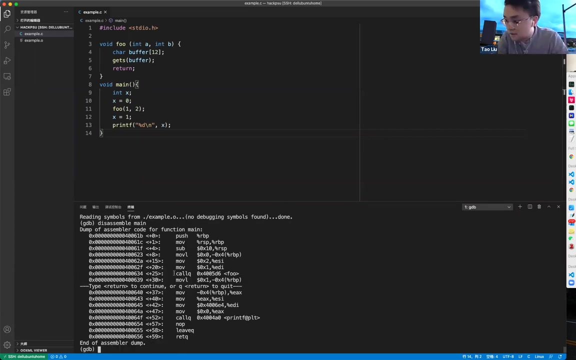 So this example. So, for example, we want to see the assembly language of the main function We can see here. So let me enlarge it So, as you can see here this instruction, want to create a. let me enlarge it So, as you can see here this instruction, want to create a. 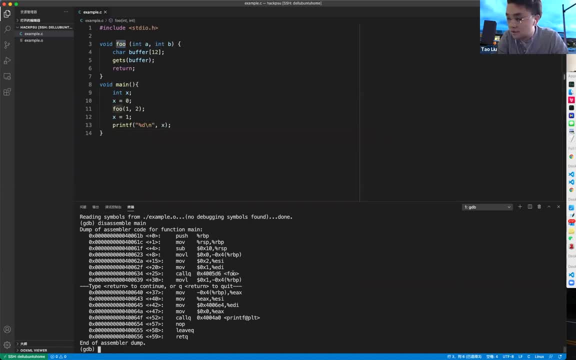 call the function, for This is the function: call instruction, And afterwards you can see this is a constant one. So basically, this instruction is trying to assign one to X. So if you want to skip this assignment, you need to skip this instruction. 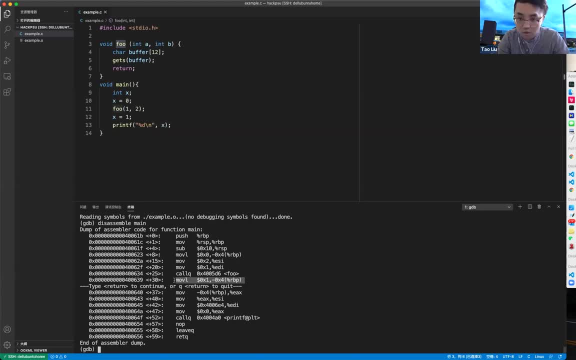 So this instruction is stored in the stack, the return address. So if you want to skip this assignment, you need to manipulate the contents of the return address So you can use some method to execute the next instruction. Basically, you need to know the offset. 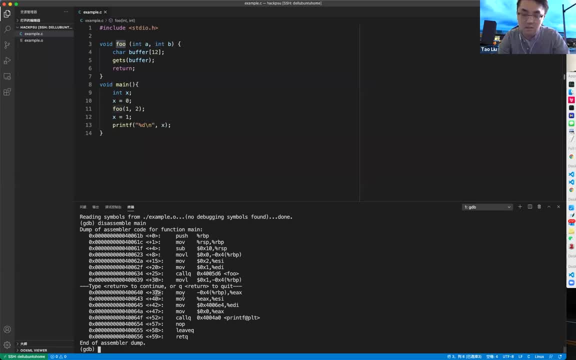 between these two instruction, which is seven. So this is what the attacker want to know, because he want to know offset, He want to know the offset. So you need to skip this instruction and execute this instruction directly. So yeah, this is how you can skip one assignment. 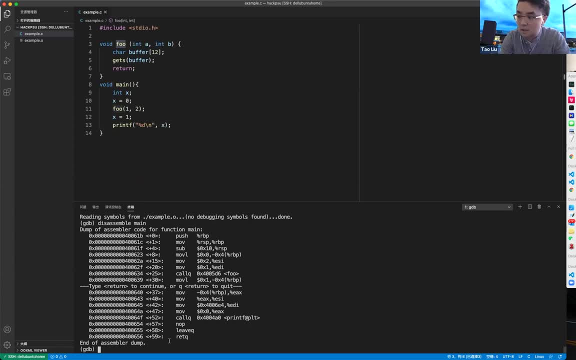 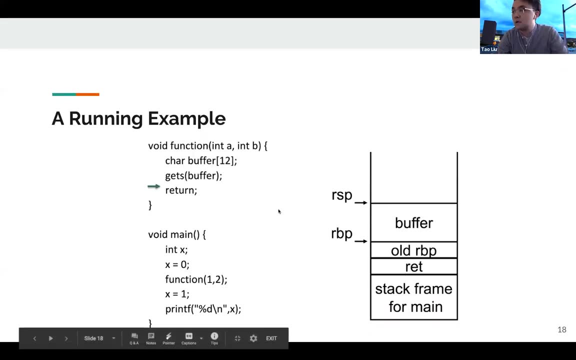 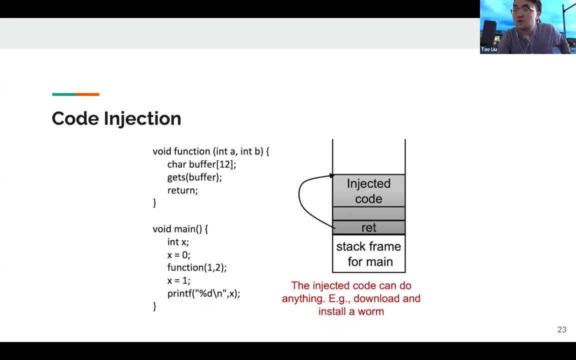 in your source code And also, I think this is enough, Let's go back to slides here. So we have, yeah, we have figured out here, and then let's see, Yeah, this is the most dangerous one. This is called the code injection. 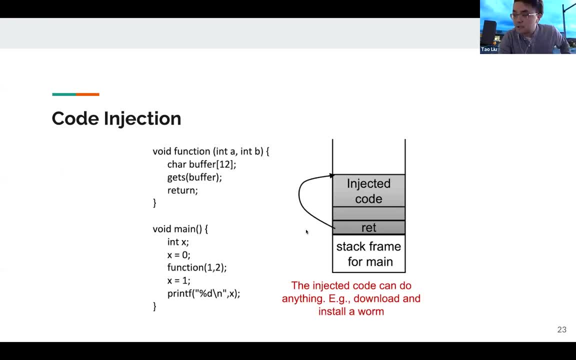 So let's see how it works. So basically, like I said, we, the attacker, want to manipulate the contents of the return address. So, for example, they know where the return address is and we assume they can manipulate that return address. Then they can put some injected code in there. 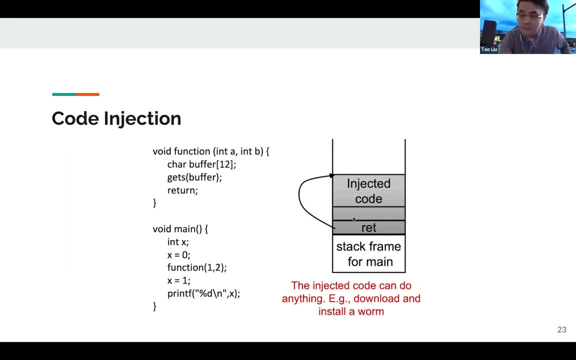 Then they can put some injected code in there. Then they can put some injected code in there, You know, in their input So they can let the return address points to the code that they want to execute it And the injected code can do anything. 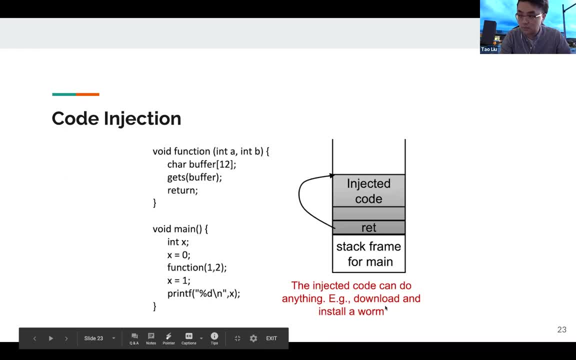 For example, download and the install a worm. So basically the code will be executed and maybe a malware or ransomware will be in store in your computer And you know you need to pay to to redeem your computer back. You need to pay some money to the attacker. 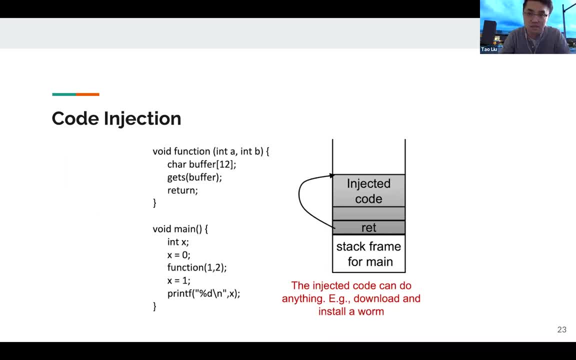 I believe some of you may know the ransomware, some malware, right? So this kind of vulnerability can be exploited by the attacker to implement some attacks. So, for example, a lot of servers, they are using the Linux system, right, And you know there are constant. 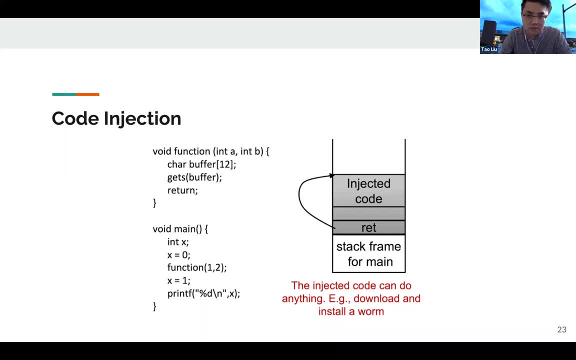 or continuous vulnerabilities are discovered in the Linux module, which is the Linux kernel, And they will, they and the such, once such vulnerabilities can be exploited by the attacker. you know, a lot of servers can be compromised And it, you know, sometimes you. 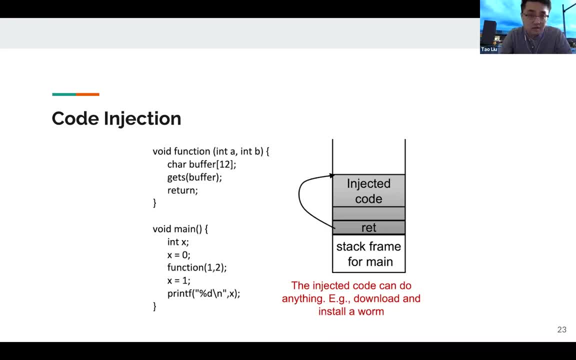 we will see. there are some events that some servers of some big companies are down, They may suffer from a cyber attack And their servers are compromised by the attacker, And the attacker can ask some money, some property from the company. So this is very serious. 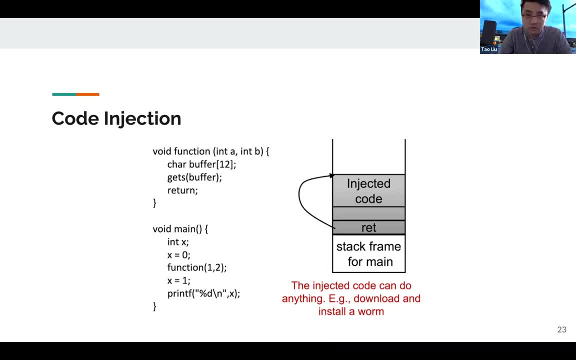 This is very severe And a lot of you know security researchers and engineers are working to defend the you know such attacks and protect our you know intelligence property, protect our property. So, yeah, This is why we should pay attention to the security. 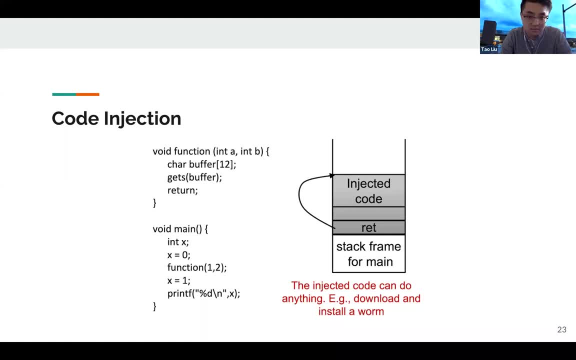 of a computer system to the IOT system. As you know, currently we are. we are having a lot of IOT devices, Not only in our life. we have a lot of IOT device in manufacturing, in the, you know, in the industrial system. 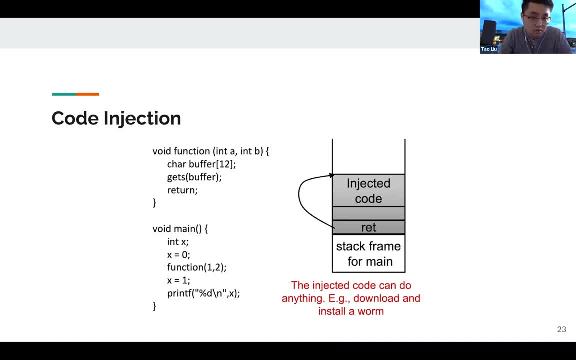 in the autonomous vehicles, right. So we have a lot of such IOT devices And we need to pay attention to the security aspect of such systems because once attacker, they found a way to exploit the system a lot of better things they can do.